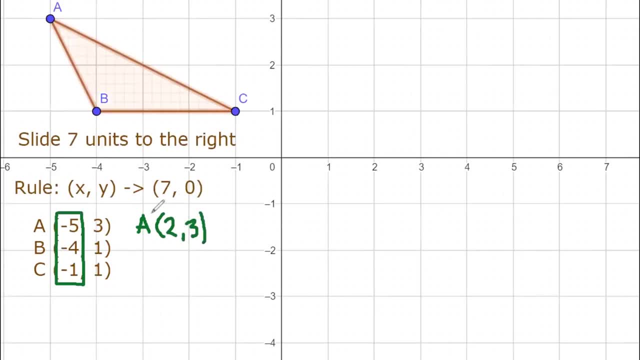 now for a is 2, 3. We call it a apostrophe or a sub 1.. Next our b: negative 4 plus 7.. And that gives you positive 3.. S: 5, 0.. You just bring down your y values. Next, for letter c, you have negative 1.. Negative: 1 plus. 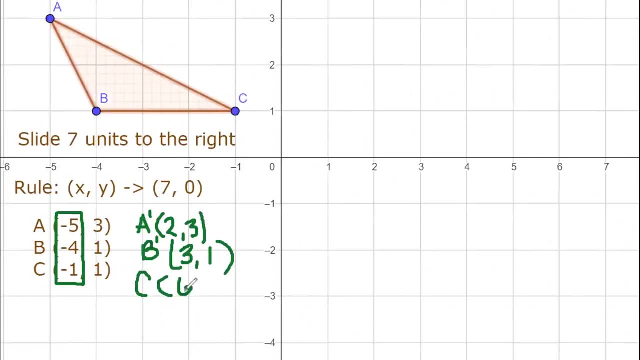 7 is positive, 6. Positive: 1. So it now. your new coordinates are: a is 2, 3. So we have: b is 3, 1. Then c is 6, 1. So next letter c, you have 1.. Negative: 1 plus 7 is positive 6.. Negative 1 plus 7 is positive 1.. negative 6: 0, positive 1. Now that we already know that we have three down this, the rightじゃあ, we'll rotating. then c, s6, one, and now let's go to d and d. 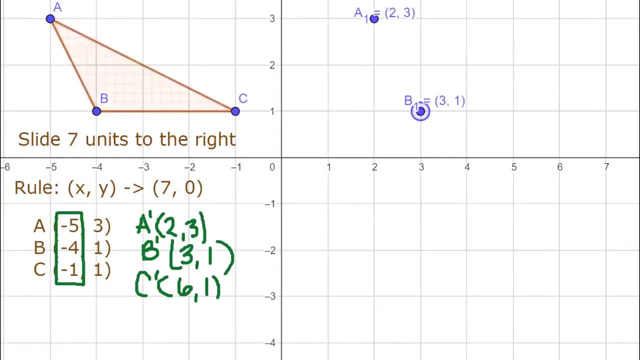 So I'll just plot it to the right: B is 3, 1,, then C is 6, 1.. After which you can connect the dots to form your triangle. Now it is translated to the right side of the coordinate plane in quadrant 1.. 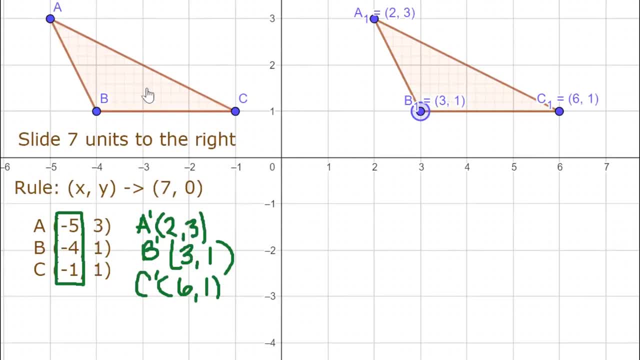 So now the object is translated to the right 7 units. So if you drag this object, 7 units 1, 2, 3, 4,, 5, 6, 7.. The object is correctly translated to the right 7 units. 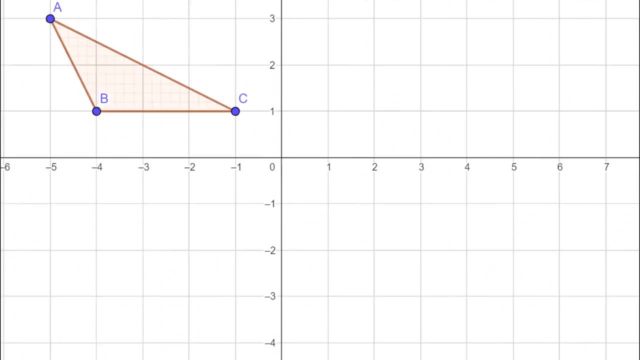 Next example: we are going to move the same triangle ABC. We are going to move downwards 4 units. So slide the image 4 units downward. So in our rule it will be written as X. Y will be changed into 0, negative 4.. 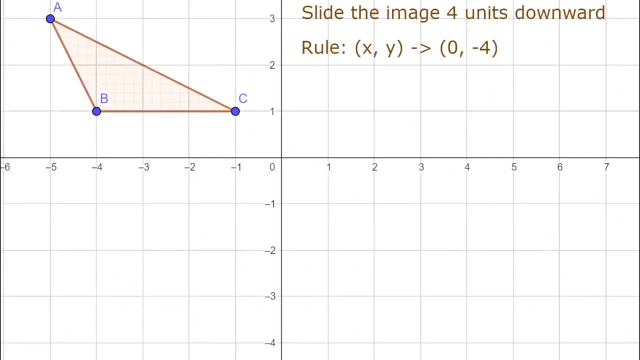 It means our Y will go down 4 units. Then the same thing, we are identifying our A, B and C coordinates. So A is negative 5, 3.. B is negative 4, 1.. C is negative 1,, positive 1.. 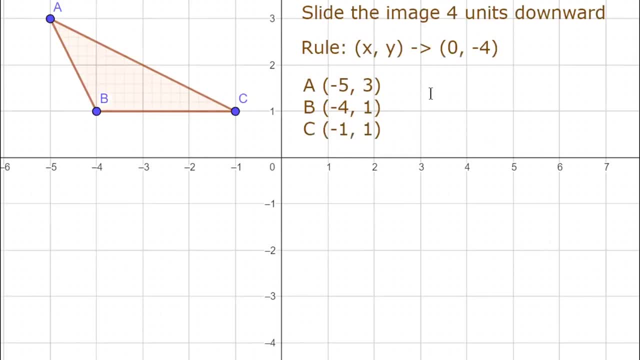 So subtracting or adding negative 4, 1, C is negative, 1, positive, 1.. Negative 4 to our Y values. What we are going to do now is to add negative 4 to our Y values. So let's do it. 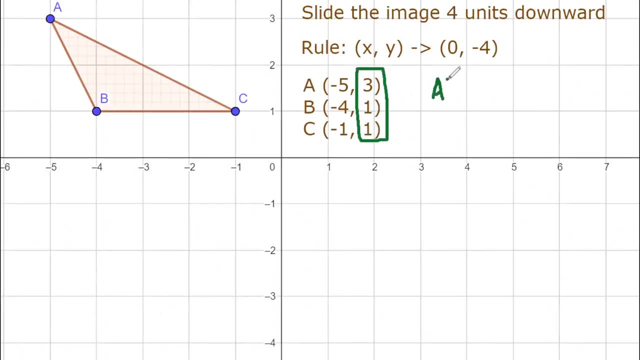 So our A sub 1 or A apostrophe will become: just copy your X, so that is negative 5. Then comma 3 minus 4 or 3 plus negative 5. So that is negative 5.. Negative 4 is negative 1.. 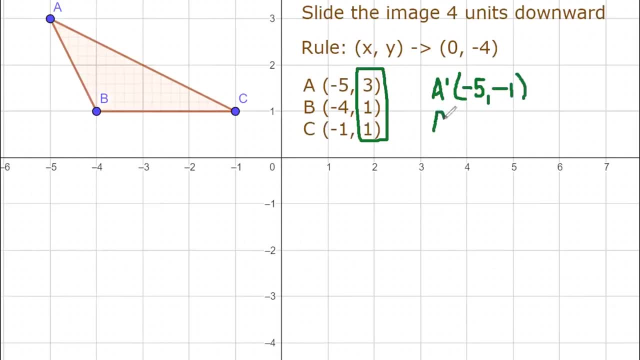 That is now your new coordinate. Next for B, B sub 1 or B apostrophe, we have negative 4.. 1 plus negative 4 is negative 3.. Then your C is equal to negative 1, comma. 1 plus negative 4 is negative 3.. 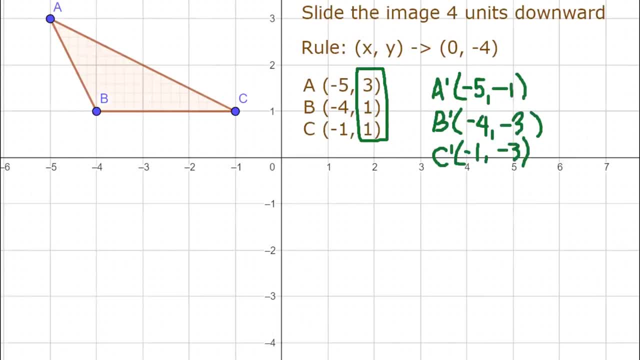 So you can find your coordinates on quadrant 3, because all are negative. So you have A sub 1, negative, 5, negative, 1.. B sub 1 is negative, 4, negative, 3.. C sub 1 is negative, 1, negative, 3.. 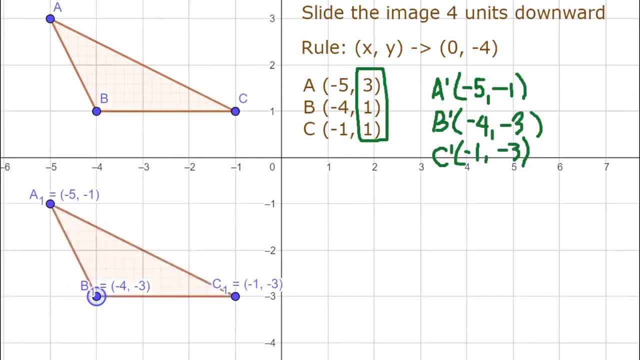 Then you can connect the dots to form the triangle ABC. So if you are going to check four units below, so from the original position you can drag the image 1, 2, 3, 4.. Exactly, the image was translated. 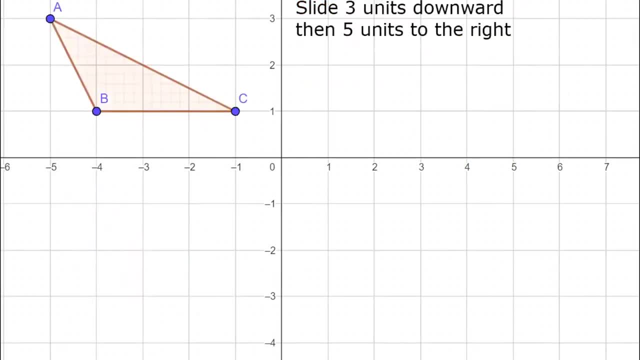 Four units downward. For the third example, we are going to move the image three units downward and five units to the right. So your rule will become X, Y plus 5 to the right and minus 3 downwards. So let's give our points. 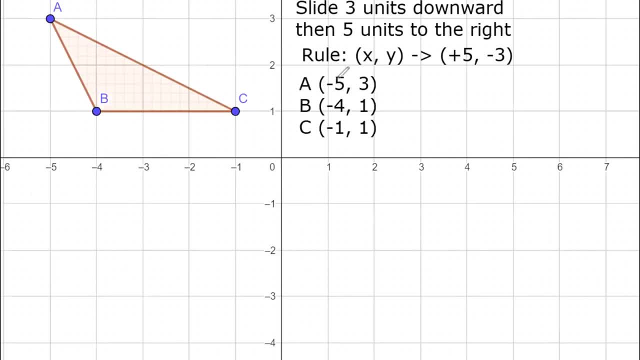 Our points are coordinates for A- negative 5, 3, B- negative 4, 1,. C- negative 1, 1.. Then what we're going to do next is to add 5 to our X values. For our A, we have negative 5 plus 5, and that gives us 0. 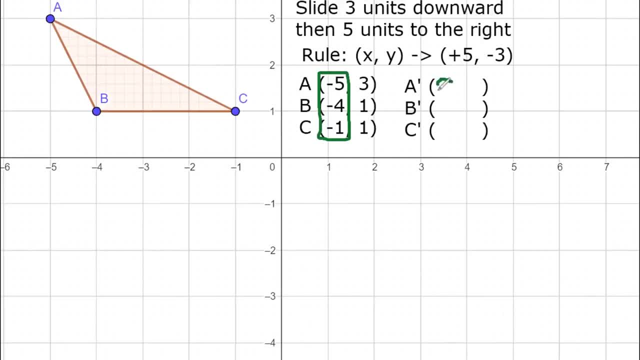 So our X in our A is 0. Then for our B, negative 4 plus 5 is 1.. And for our C, negative 1 plus 5 is positive 4.. Okay, So what we're going to do next is to find our coordinate for Y. Y is 3 minus 3..